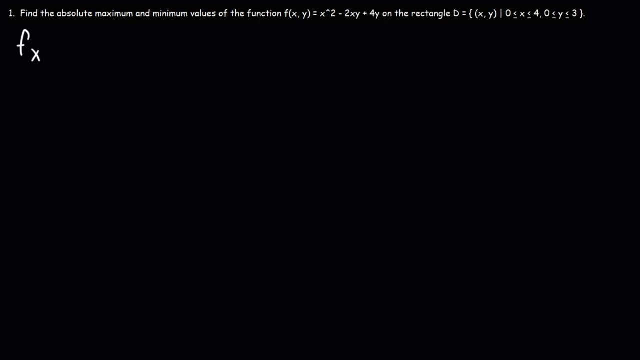 the partial derivative with respect to x and with respect to y. So let's find f sub x first. The derivative of x squared is 2x. The derivative of negative: 2xy. that's going to be negative 2 times the derivative of x, which is 1, times y, So that becomes negative 2y. 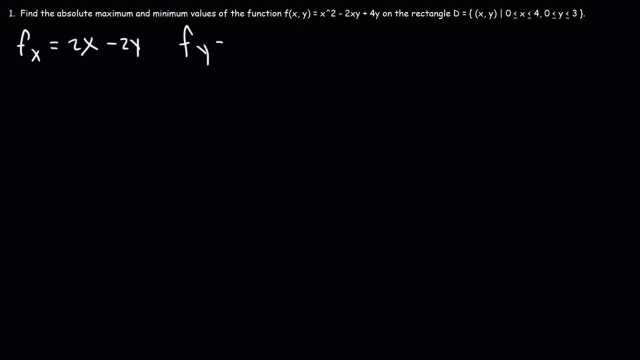 Now the partial derivative with respect to y is going to be the derivative of x, squared becomes 0, the derivative of negative 2xy. it will be negative 2x times the derivative of y, which is 1.. So that's negative 2x And the derivative of 4y will just be 4.. 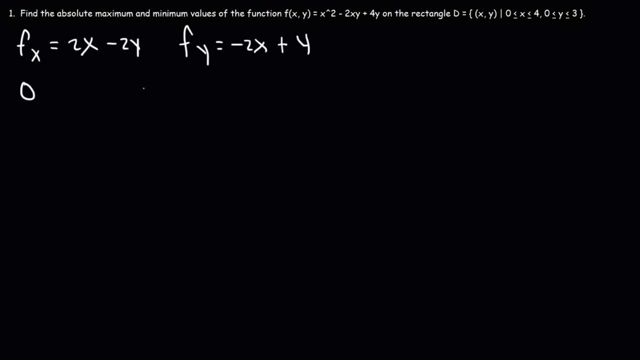 Now our next step is to set each partial- excuse me, each partial- derivative equal to 0. And we want to solve for x and y. On the left, we could take out a 2.. On the right, we could take out a negative 2, which will leave behind x minus 2.. 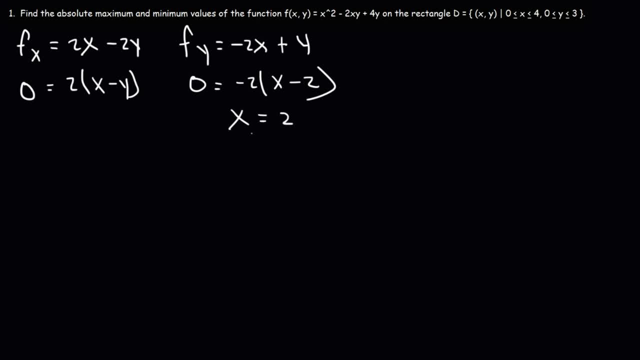 So we could solve for x here x is 2.. Now if we take that x value, plug it into that expression, we can see that y is equal to 2.. So this gives us the critical point, 2 comma 2.. 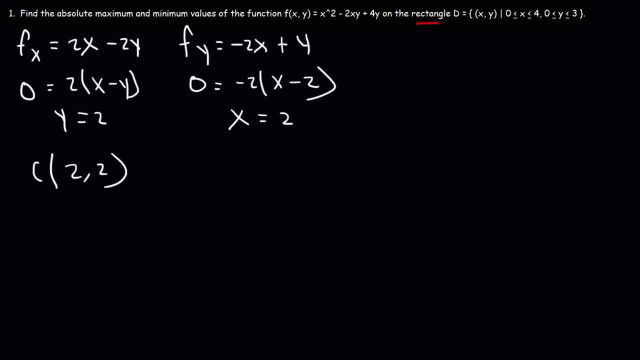 Now, what I'm going to do is I'm going to draw the rectangle bounded by x and y. So here is the rectangle D. It has the points 0, 0,, 4, 0.. These are the endpoints of the rectangle. 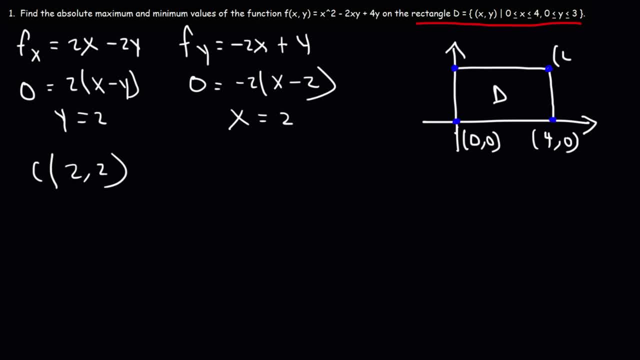 y varies from 0 to 3, so this point must be 4 comma 3.. And over here this is 0 comma 3.. Now you want to break up the rectangle into four line segments, So we're going to call this L1, L2, L3, and L4. 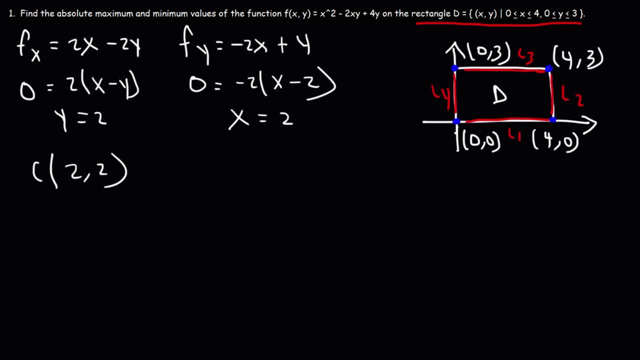 Now the absolute maximum and minimum values could be any one of the four endpoints that we have on this rectangle. It could be a point on the line segment. It could be this critical point. It could be a point here or some other point inside this region. 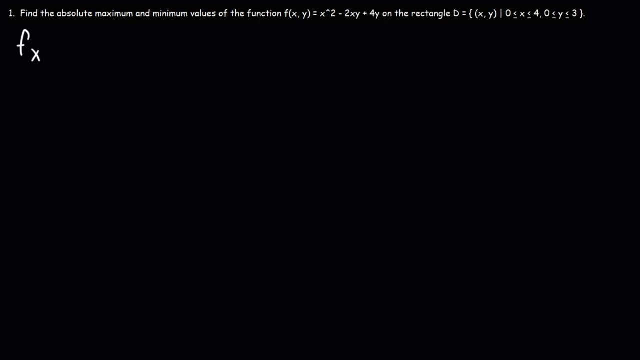 the partial derivative with respect to x and with respect to y. So let's find f sub x first. The derivative of x squared is 2x. The derivative of negative: 2xy. that's going to be negative 2 times the derivative of x, which is 1, times y, So that becomes negative 2y. 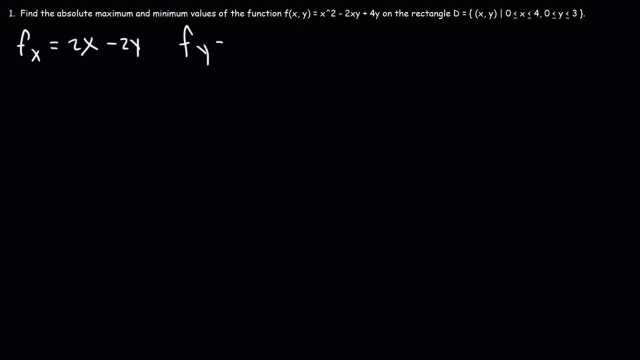 Now the partial derivative with respect to y is going to be the derivative of x, squared becomes 0, the derivative of negative 2xy. it will be negative 2x times the derivative of y, which is 1.. So that's negative 2x And the derivative of 4y will just be 4.. 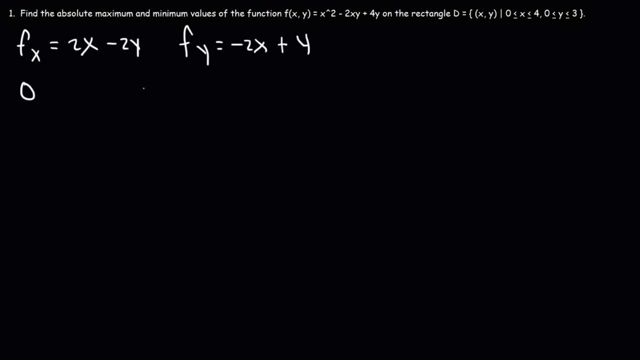 Now our next step is to set each partial- excuse me, each partial- derivative equal to 0. And we want to solve for x and y. On the left, we could take out a 2.. On the right, we could take out a negative 2, which will leave behind x minus 2.. 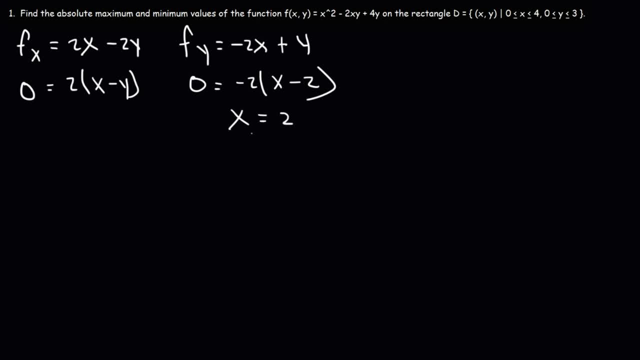 So we could solve for x here x is 2.. Now if we take that x value, plug it into that expression, we can see that y is equal to 2.. So this gives us the critical point, 2 comma 2.. 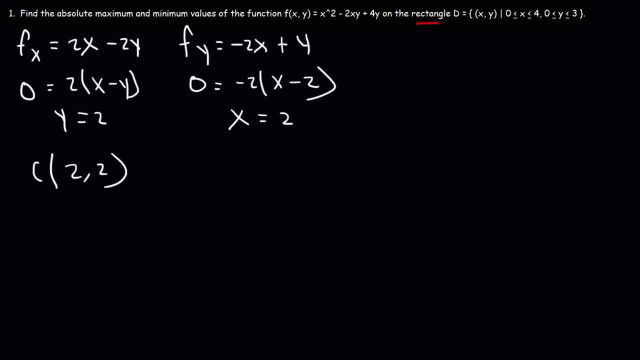 Now, what I'm going to do is I'm going to draw the rectangle bounded by x and y. So here is the rectangle D. It has the points 0, 0,, 4, 0.. These are the endpoints of the rectangle. 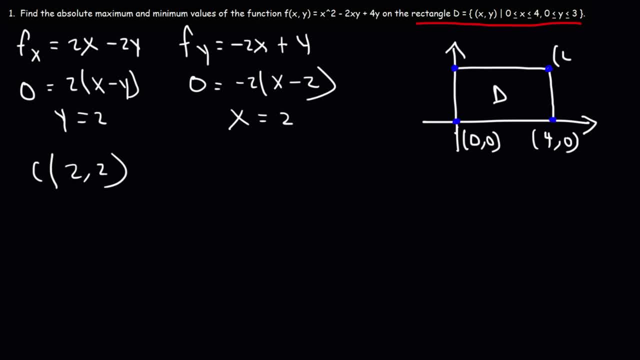 y varies from 0 to 3, so this point must be 4 comma 3.. And over here this is 0 comma 3.. Now you want to break up the rectangle into four line segments, So we're going to call this L1, L2, L3, and L4. 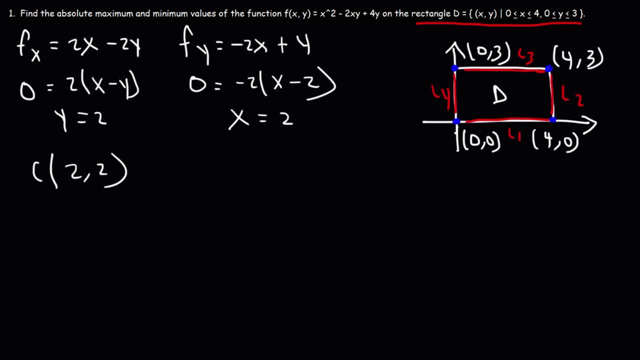 Now the absolute maximum and minimum values could be any one of the four endpoints that we have on this rectangle. It could be a point on the line segment. It could be this critical point. It could be a point here or some other point inside this region. 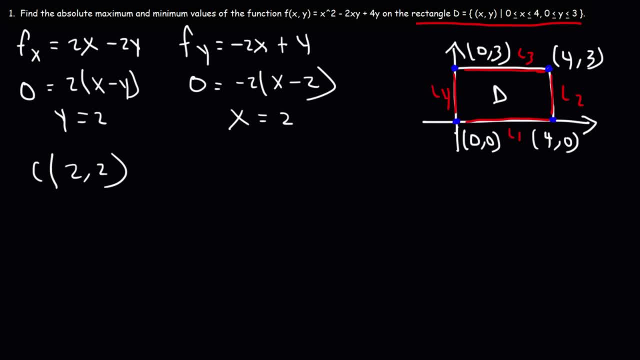 But we have to find out where those points are. Now. one thing that we need to do is make sure that the critical point lies in the rectangle D, which it does. 2 comma 2 is definitely in this range. So now the next thing I'm going to do is make a table with x, y and the function value f. 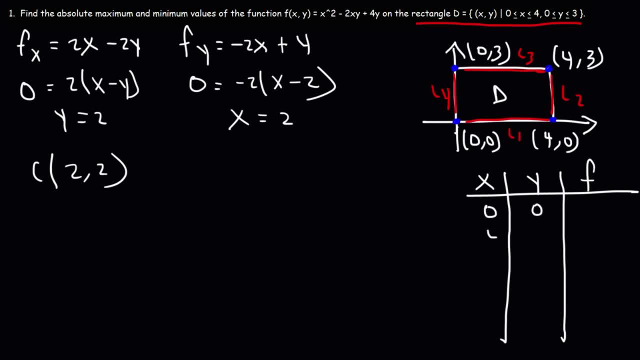 And I'm going to place all of the endpoints in this table, as well as the critical point 2, comma 2.. Now let's focus on the first line, segment L1.. In this line segment we can see that x, or rather y, is always equal to 0. 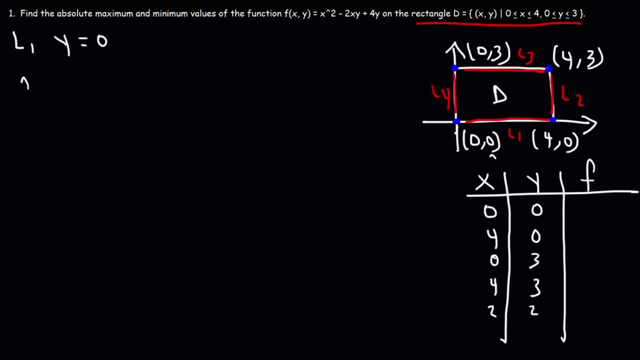 So we have the function f of x, comma 0. I replaced y with 0. And that's going to be x squared minus 2x times 0 plus 4 times 0. So we have the function x squared. 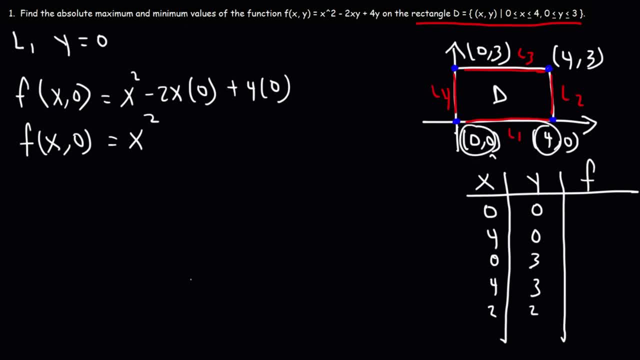 And this is going to be between 0 and 4.. Between 0 and 4, x squared is an increase in function. So for this function, 0 is going to give us a minimum value, 4 is going to give us a maximum value. 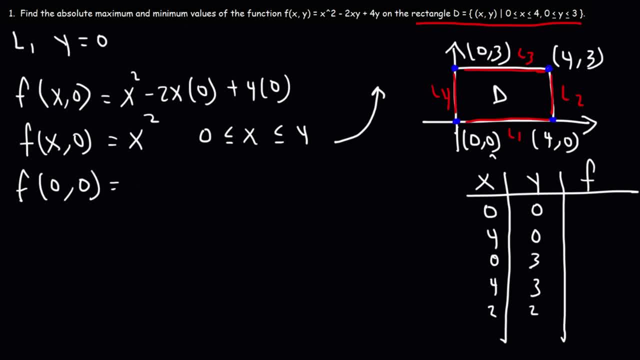 So if we replace x with 0,, we'll get 0 squared, which is 0.. If we replace x with 4, we'll get 4 squared, which is 16.. And now we could put these values in this table. 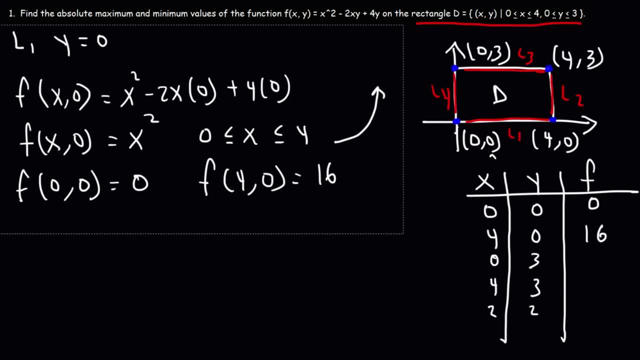 So that's it for line segment, Or we could say just segment 1.. Now let's move on to segment 2, L2.. So notice that x doesn't change. So for this segment x is always 4.. 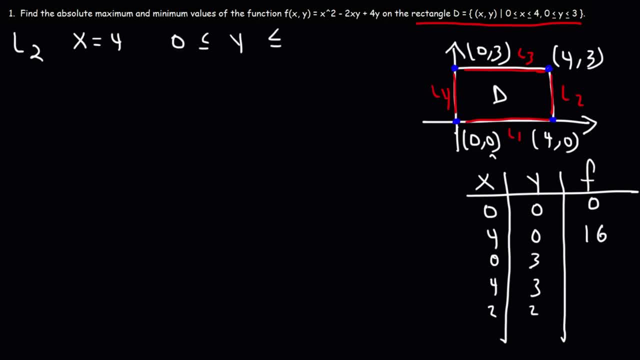 Y varies between 0 and 3 for that line segment. Now let's plug in 4 into this function. So this is going to be f 4 comma y. So replacing x with 4, we're going to have 4 squared minus 2 times 4 times y plus 4y. 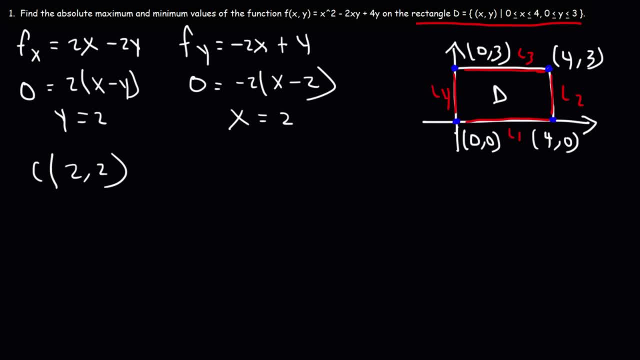 But we have to find out where those points are. Now. one thing that we need to do is make sure that the critical point lies in the rectangle D, which it does. 2 comma 2 is definitely in this range. So now the next thing I'm going to do is make a table with x, y and the function value f. 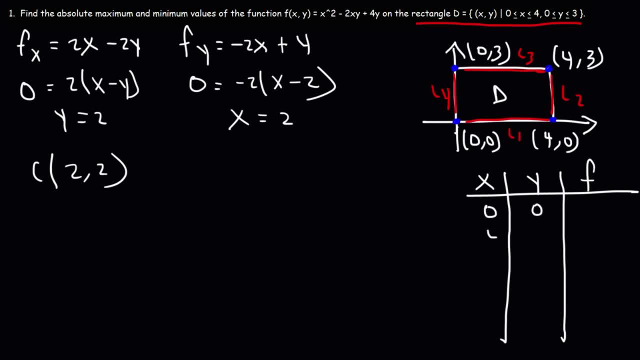 And I'm going to place all of the endpoints in this table, as well as the critical point 2, comma 2.. Now let's focus on the first line, segment L1.. In this line segment we can see that x, or rather y, is always equal to 0. 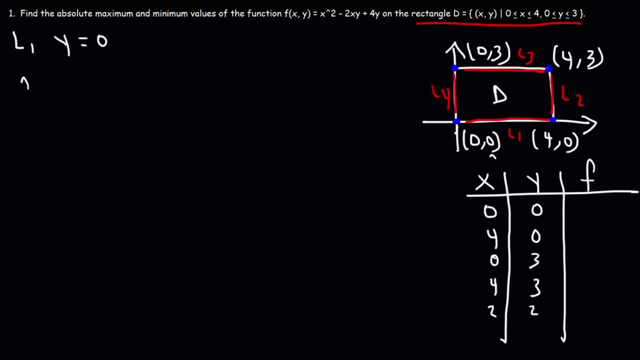 So we have the function f of x, comma 0. I replaced y with 0. And that's going to be x squared minus 2x times 0 plus 4 times 0. So we have the function x squared. 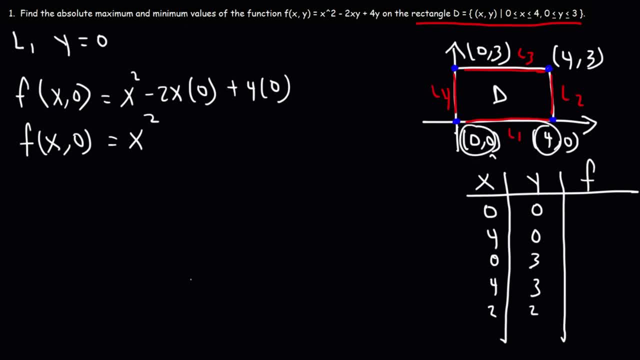 And this is going to be between 0 and 4.. Between 0 and 4, x squared is an increase in function. So for this function, 0 is going to give us a minimum value, 4 is going to give us a maximum value. 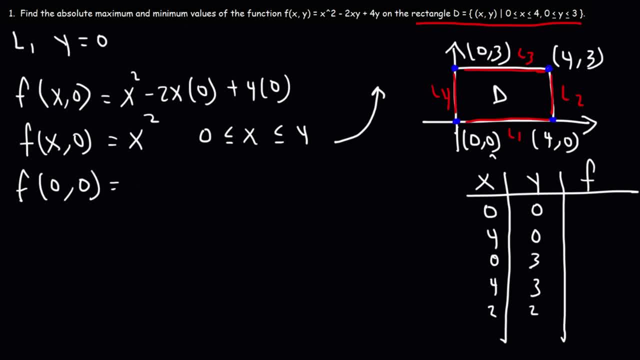 So if we replace x with 0,, we'll get 0 squared, which is 0.. If we replace x with 4, we'll get 4 squared, which is 16.. And now we could put these values in this table. 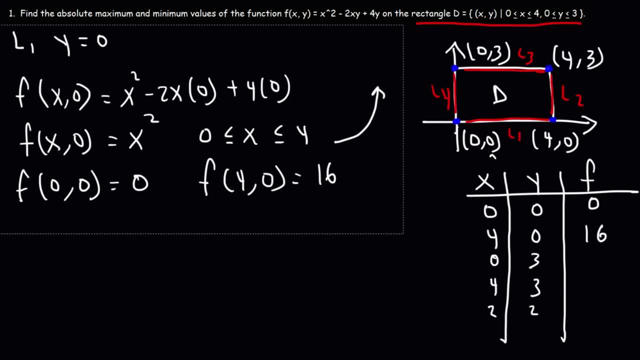 So that's it for line segment, Or we could say just segment 1.. Now let's move on to segment 2, L2.. So notice that x doesn't change. So for this segment x is always 4.. 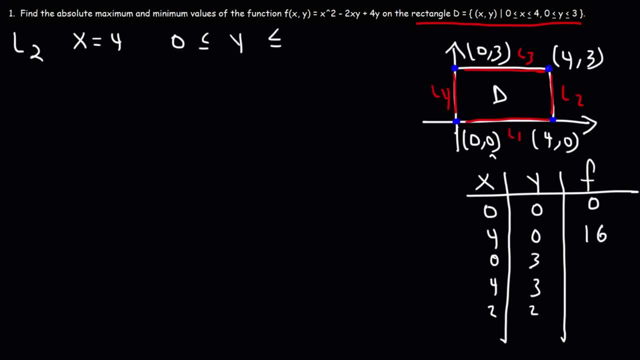 Y varies between 0 and 3 for that line segment. Now let's plug in 4 into this function. So this is going to be f 4 comma y. So replacing x with 4, we're going to have 4 squared. 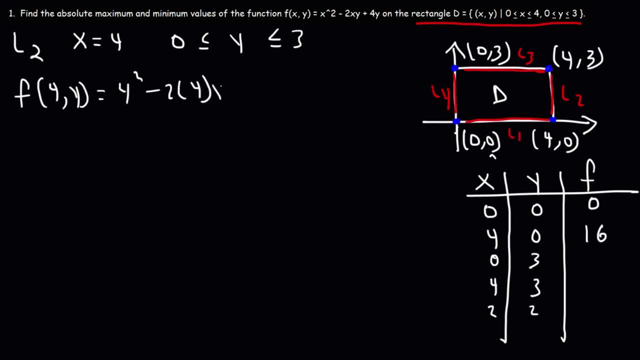 minus 2 times 4 times y plus 4y, So that's 16 minus 8y plus 4y, which becomes 16 minus 4y. So this is a linear function and it's a decrease in function. 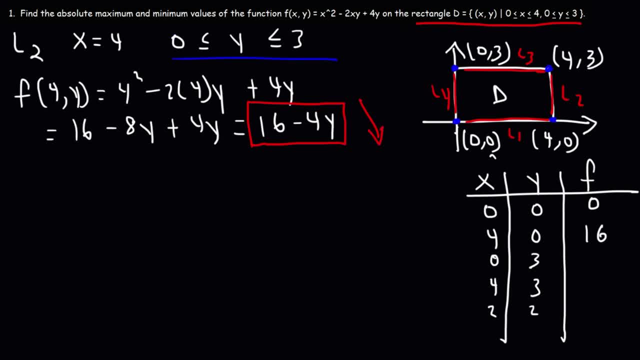 So, On the interval from 0 to 3, y equals 0 will be a maximum value, and y equals 3 will be a minimum value, since it's always decreasing, So let's plug in 0 first. So this will be 16 minus 4 times 0, which is 16.. 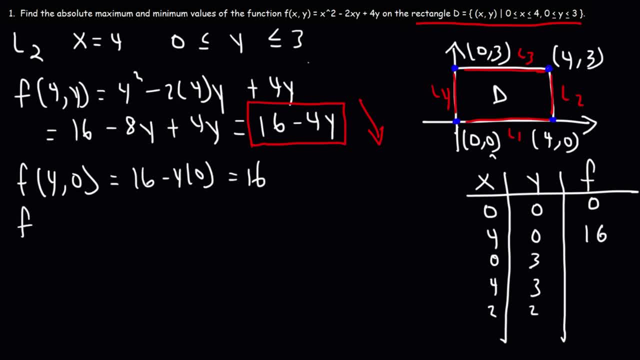 And we already have that value. Now let's replace y with 3.. So this will be 4, 3.. And so it's going to be 16 minus 4 times 3. That's 16 minus 12,, which is 4.. 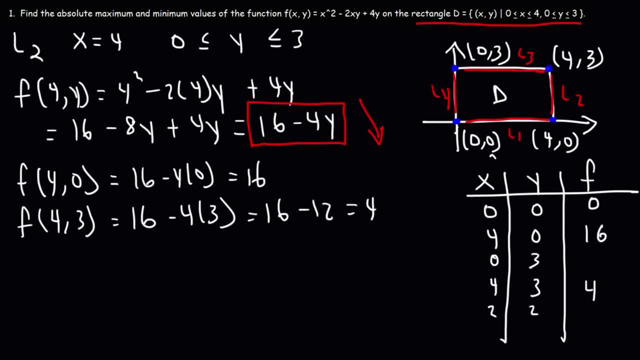 So that's a new value that we can put there. And that's it for line segment 2.. Now let's move on to line segment 3.. So for this one, we can see that y is always 3.. And we can see that y is always 3.. 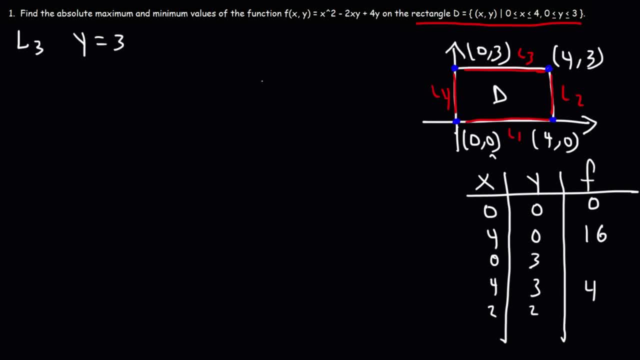 And we can see that y is always 3.. And we can see that x varies between 0 and 4.. So, replacing y with 3, we have f of x, 3. That's going to be x squared minus 2x times 3, plus 4 times 3.. 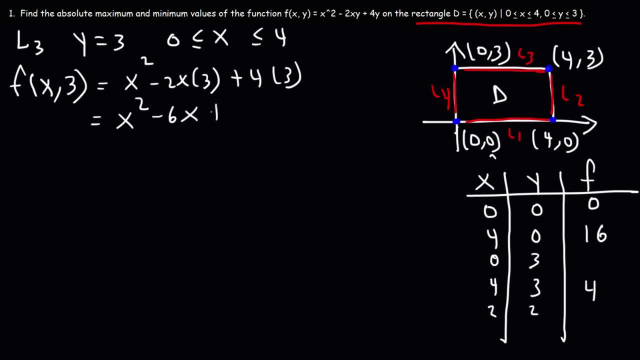 So that's x squared minus 6x plus 12.. So this is a parabolic function. So this is a parabolic function like this. We're going to plug in 0 first, So this will be f of 0, 3.. 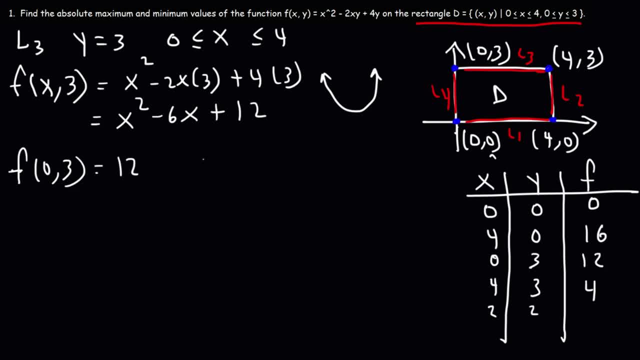 And that's going to be 12, which we can put here, And then we're going to plug in 4.. So f of 4, 3.. Notice that we already know what that is. That's equal to 4.. 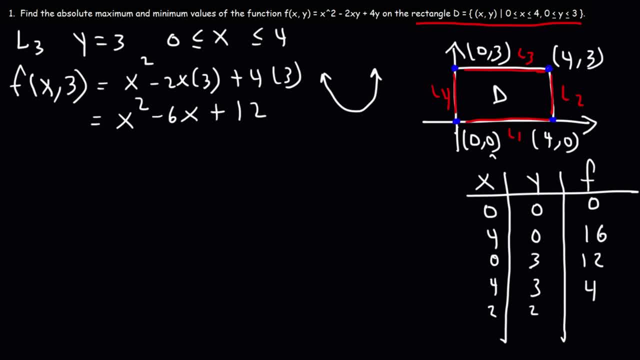 Now, because we have a quadratic expression, we know that there's a minimum value somewhere And to find it we could find the first derivative of this expression. So f, prime of x, 3, that's going to be 2x minus 6.. 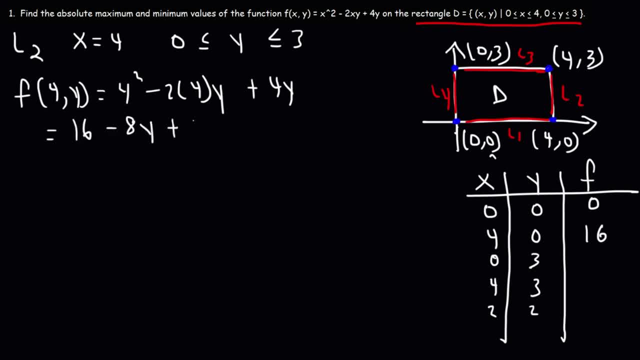 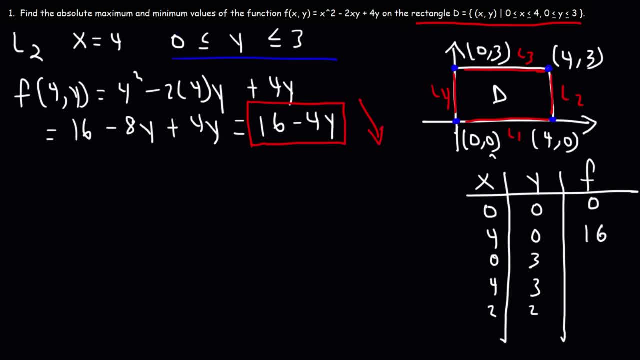 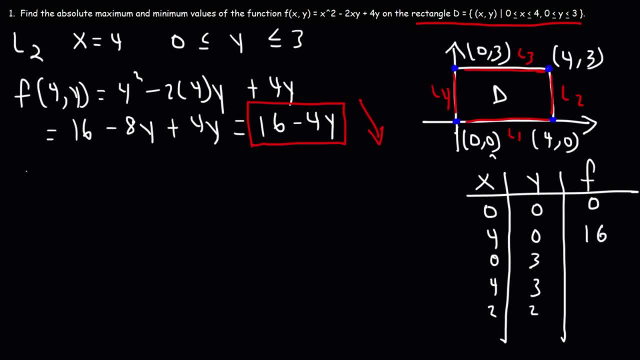 always decreasing, So let's plug in 0 first. So this will be 16 minus 4 times 0, which is 16, and we already have that value. Now let's replace y with 3.. So this will be 4 comma 3.. 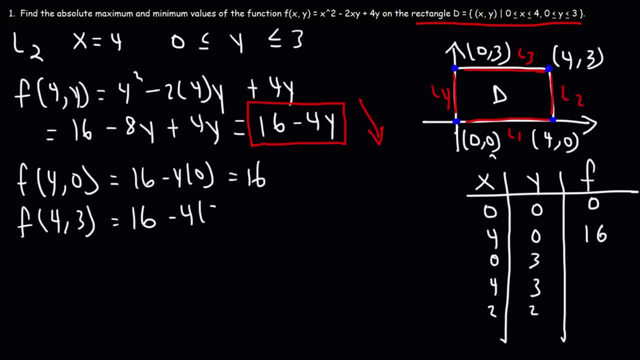 3, and so it's going to be 16 minus 4 times 3. that's 16 minus 12, which is 4. so that's a new value that we can put there. and that's it for line segment 2. now let's move on to line segment 3. so for this one we could see that Y is always. 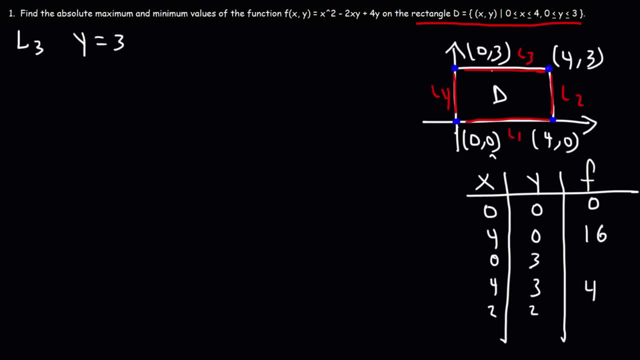 3 and we can see that X varies between 0 and 4. so, replacing Y with 3, we have F of X comma 3. that's going to be x squared minus 2x times 3 plus 4 times 3, so that's x squared minus 6x plus 12. 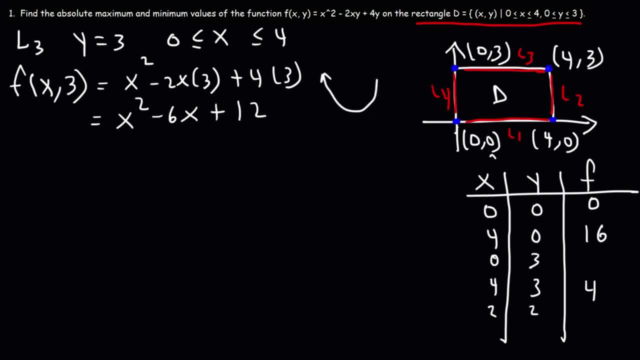 so this is a parabolic function like this: we're going to plug in 0 first, so this will be F of 0 comma 3, and that's going to be 12, which we can put here, and then we're going to plug in 4, so F of 4 comma 3. notice that we already know what. 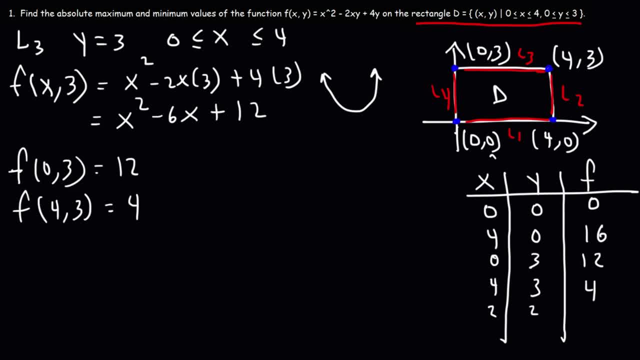 that is, that's equal to 4. now, because we have a quadratic expression, we know that there's a minimum value somewhere and to find it we could find the first derivative of this expression. so F, prime of x comma 3, that's going to be 2x minus 6, setting it. 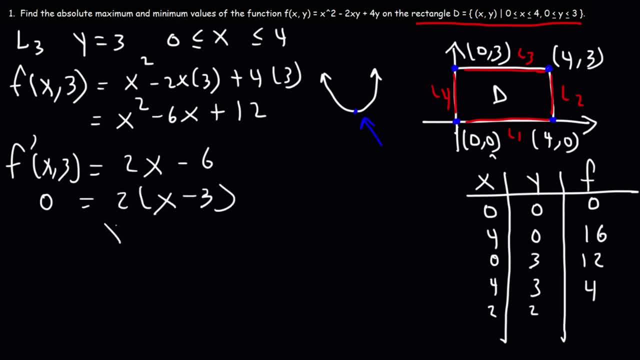 equal to 0, we can see that we have a point of interest at x equals 3. so that's we want to evaluate the function when x is 3 and y is still 3. so we have a new point that we can add in this. 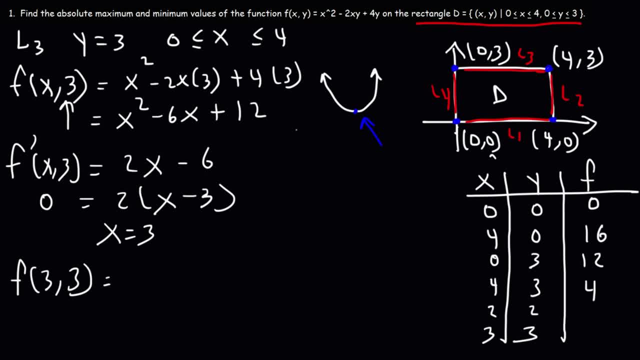 table 3 comma 3. so using this expression is going to be 3 squared minus 6 times 3 plus 12. so that's 9 minus 18 plus 12. 9 minus 18 is negative, 9 negative. 9 plus 12 is 3. now it's good to check to make sure that this point is in the 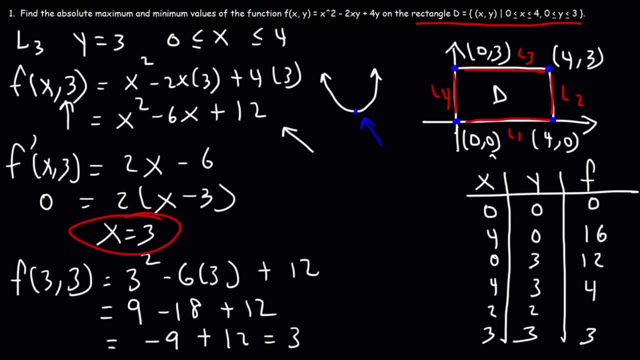 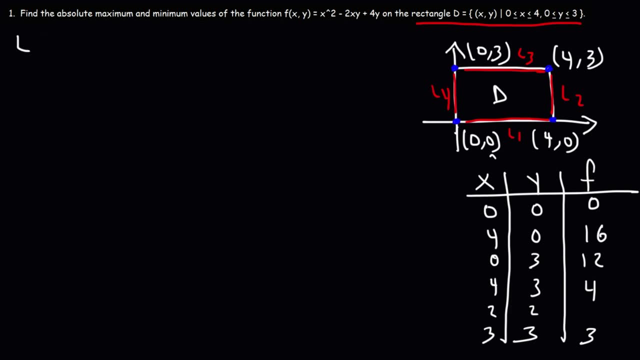 rectangular region D and 3 is definitely between 0 and 4, so it's in the range. if it's not, we would have to get rid of this value. so it's important to check that before placing it in the table. now let's move on to the fourth. 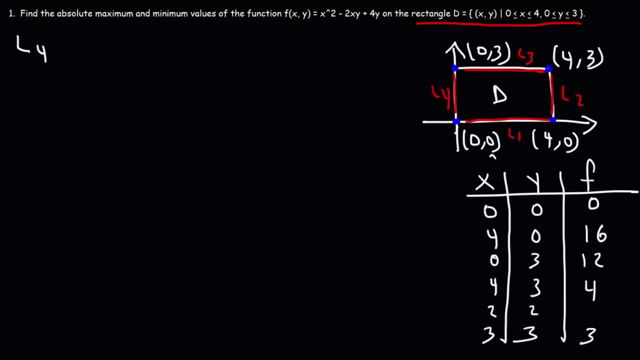 segment L4. so for this one we can see that x is equal to 0. let's move on to the next one. we could also see that y varies between 0 and 3. so we're going to replace x with 0. so we have F of 0 comma y. that's going to be 0 squared minus 2 times 0. 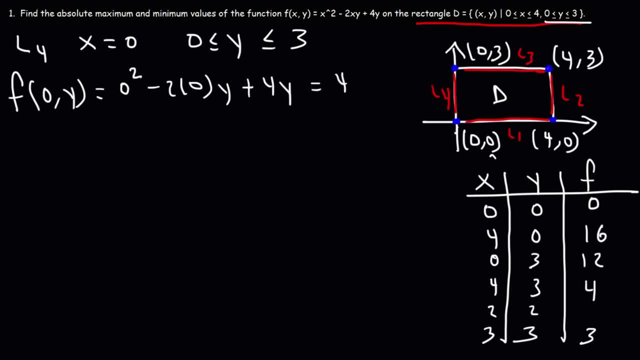 times y plus 4y, so this becomes 4y, and 4y is an increase in function. so 0 is going to give us the minimum value for 4y and 3 will give us the maximum value. so we had a 3 again. so if we go back to our equation and we put this: 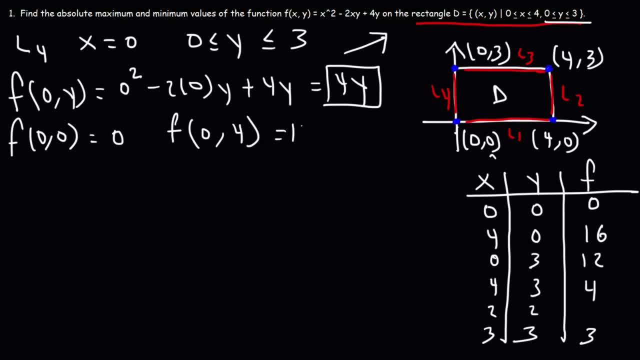 variable book out, or us. we give us that formula. let's take a look. so now we Book out: what formula is this formula? I did not got the formula for this one because I put in that here and arrow stick your object, so we're going to take these all. 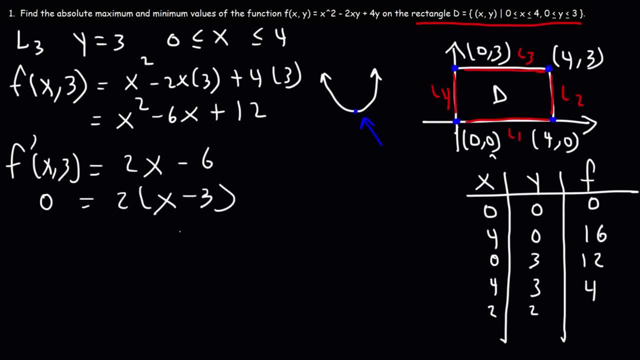 Setting it equal to 0, we can see that we have a point of interest at x equals 3.. So thus we want to evaluate the function when x is 3 and y is still 3.. So we have a new point that we can add in this table 3, 3.. 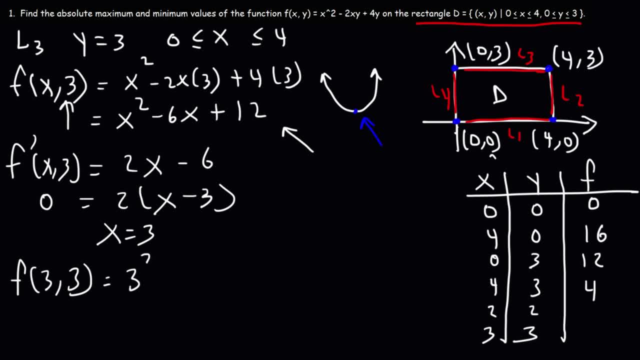 So, using this expression, it's going to be 3 squared minus 6 times 3 plus 12.. So that's 9 minus 18 plus 12.. 9 minus 18 is negative, 9.. Negative 9 plus 12 is 3.. 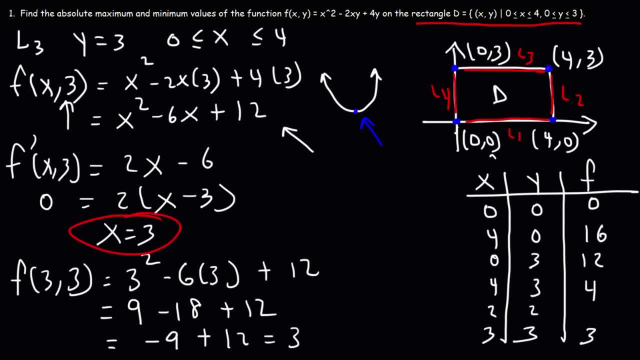 Now let's get to check to make sure that this point is in the rectangular region D, And 3 is definitely between 0 and 4. So it's in the range. If it's not, we would have to get rid of this value. 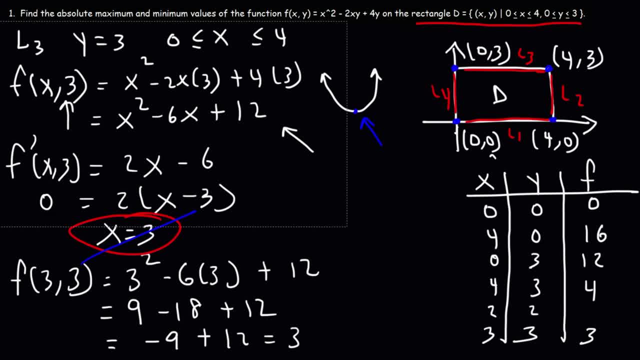 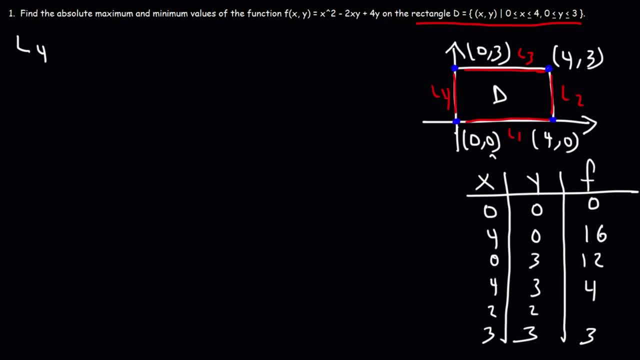 So it's important to check that before placing it in the table. Now let's move on to the fourth segment, L4.. So for this one, we can see that x is equal to 0.. We could also see that y varies between 0 and 3.. 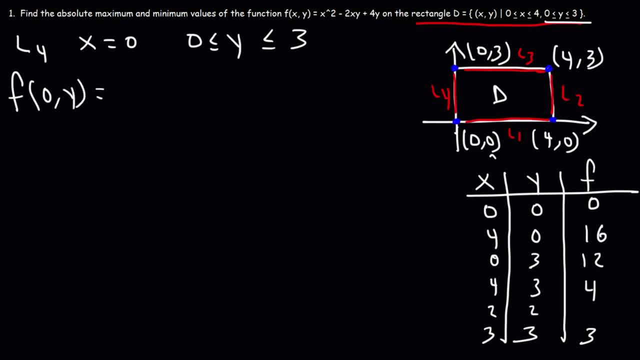 So we're going to replace x with 0.. So we have f of 0 comma y. That's going to be 0 squared minus 2 times 0, times y plus 4y, So this becomes 4y, And 4y is an increase in function. 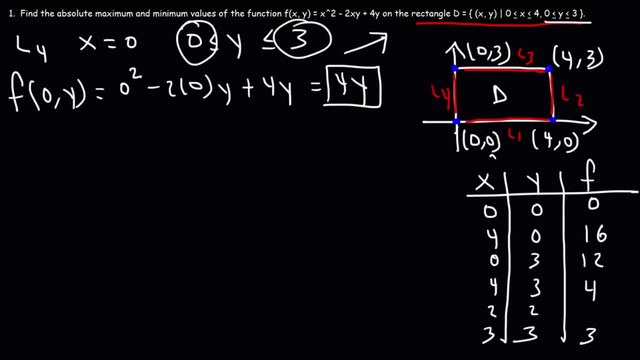 So 0 is going to give us the minimum value for 4y and 3 will give us the maximum. So when y is 0, we have f of 0, 0, which is 0.. And when y is 0,, we have f of 0, 0, which is 0. 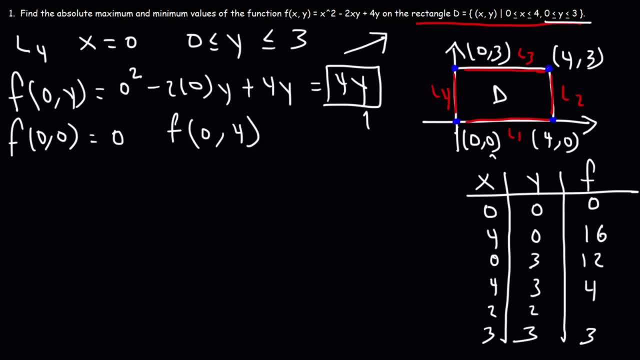 And when y is 0, we have f of 0, 0, which is 0. And when y is 4, this is just going to be 4 times 4,, which is 16.. Actually, that's supposed to be a 3 instead of 4.. 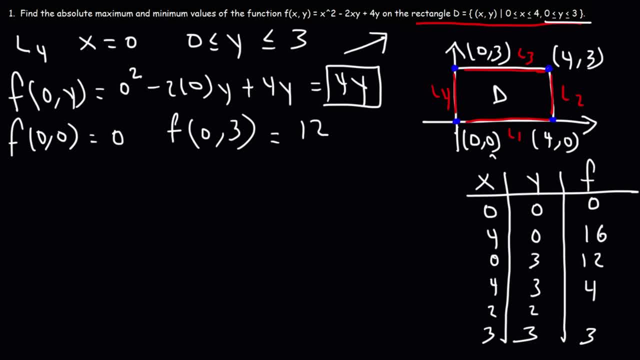 I plugged in the wrong number, So it's 4 times 3,, which is 12.. And we already have that, So there's nothing new with this segment. The only thing that we could do is plug in the critical point 2 comma 2 into the original function.